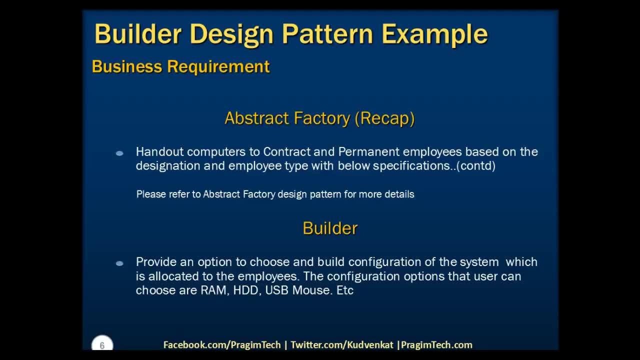 Computers to the contracts, abstract and permanent employees based on the employee type, by leveraging on specific set of rules during the employee creation. If you have not gone through the abstract factor example, we request and encourage you to view the tutorial before proceeding. Now let's consider a business requirement where a company provides an option to build 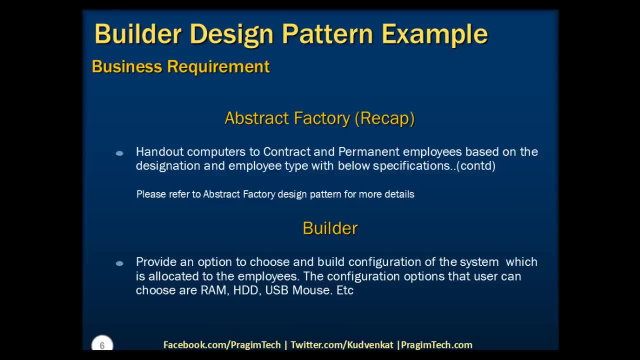 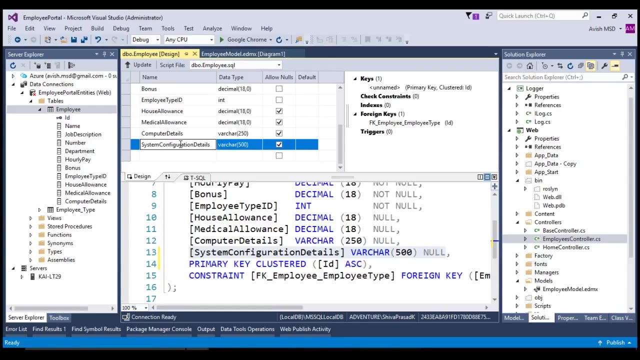 the configurations of the system which is allocated to the employees. Now let's open the visual studio and bring up the employee portal application that we have been using in the previous sessions. First, we need to create a column that holds the employee system configuration details. 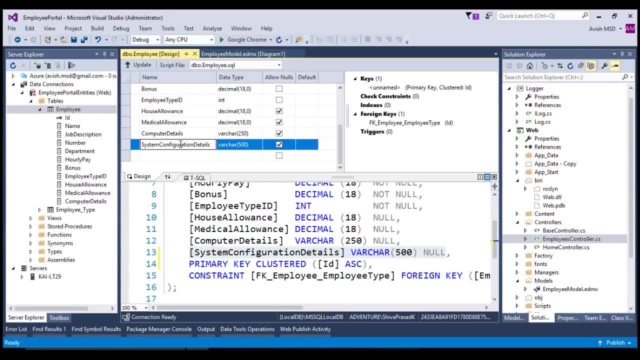 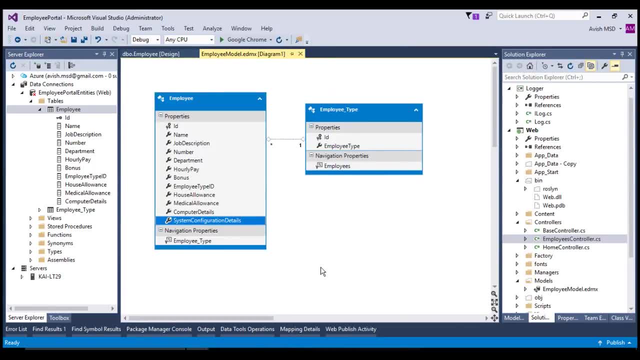 To make things faster, I have already added system configuration detail column to the employee table and I have updated this employee-modeledmx file to reflect the latest changes. Also, it's not mandatory that you need to create single column to store the entire system configuration. 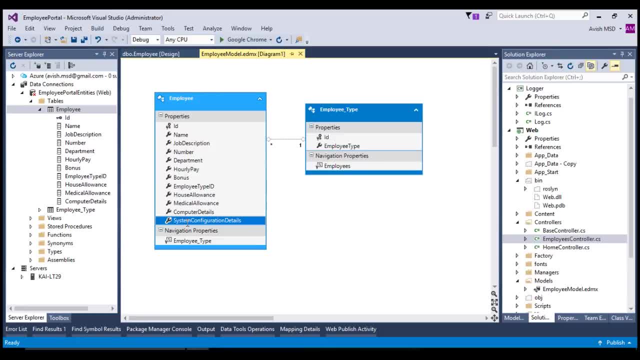 details. Based on the requirement, we can further normalize this table structure. However, I have opted to create a single column to simplify the scope of this tutorial. For more details on normalization, please refer to our SQL Server tutorials. Let's now proceed with our next step. 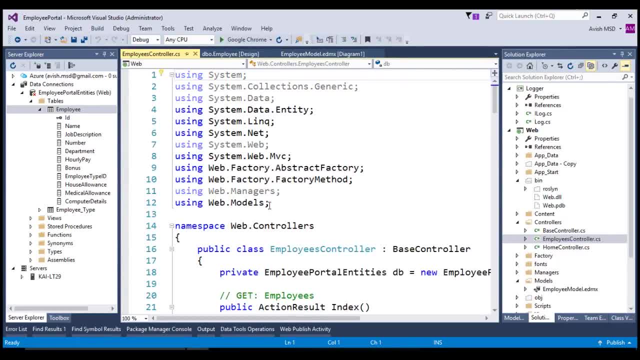 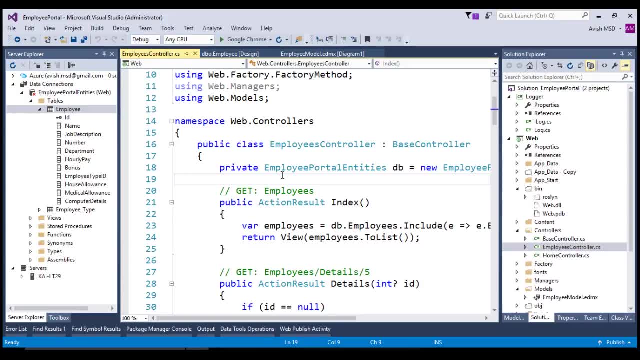 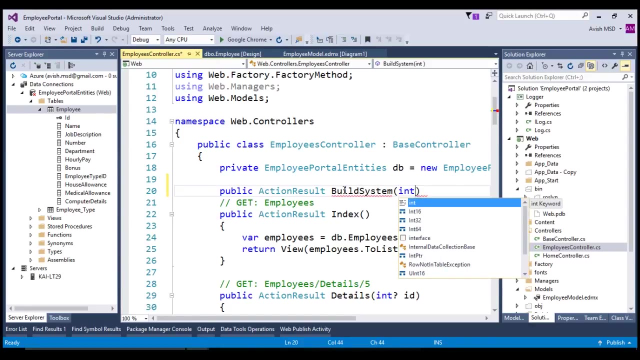 Let's open the employees controller. Let's open the employees controller And add an action method to provide an ability to choose configurations to build a system. Let's add an action method: public action research. Let's call this method as build system which access input parameter as employee ID. 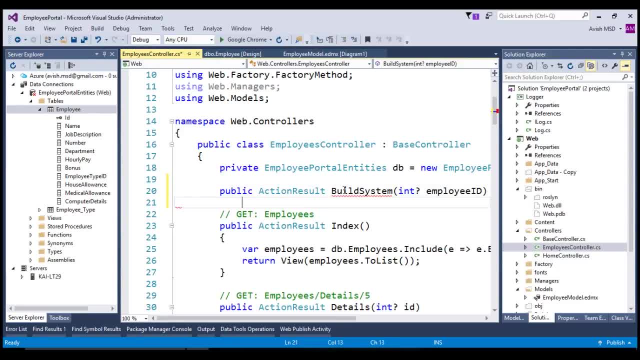 which accepts input parameter as employee ID. With need in our current程ian we can easily give a public token name Before doing ask. in the package Inuelle we have defined that useInno hash앱. We have also개� 좋아요 in our particular endpoint to check the functionality. 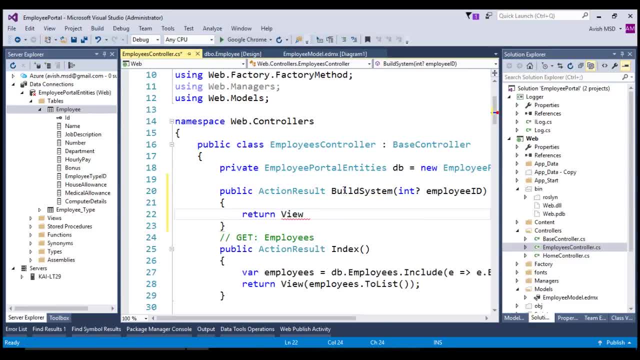 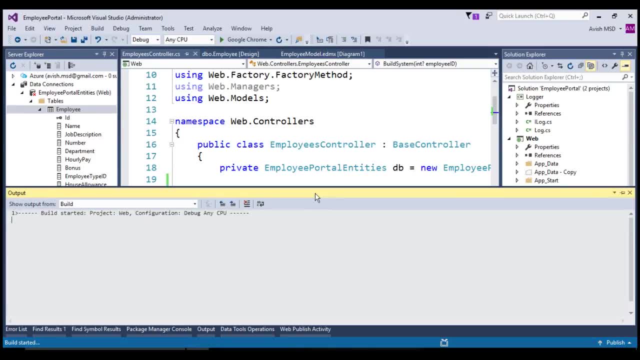 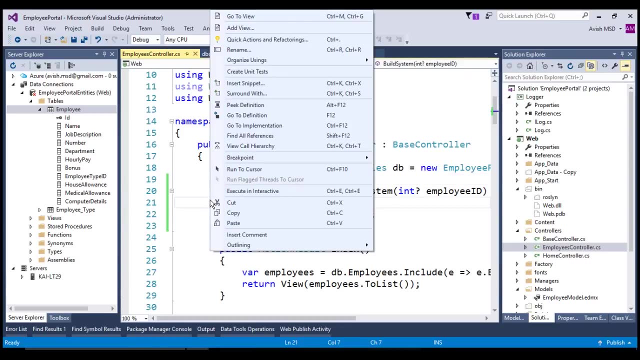 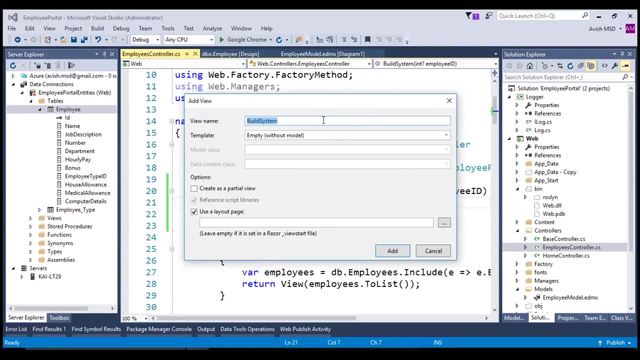 Now let's use data对 Cit proprietary. Let's return a view by passing this employee ID. Let's compile this application. Let's right click on this controller method and choose add view. Let's name this view as build system. Let's click on add. 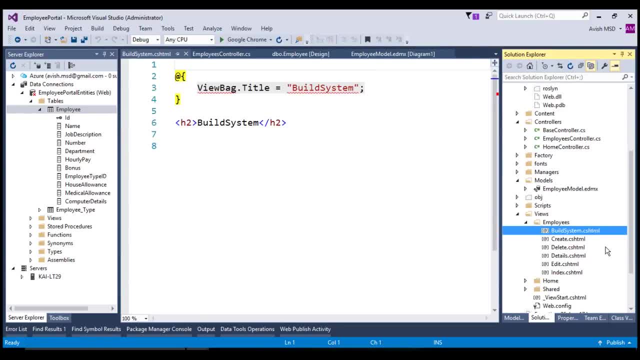 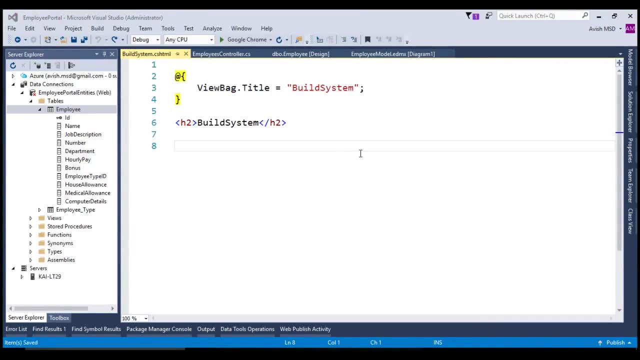 Notice that it has created a new view called build system under employees folder, Based on the requirement. let's say we need to give an ability to choose memory and hard disk size while configuring the system. I have already created the code related to the view in my notepad. 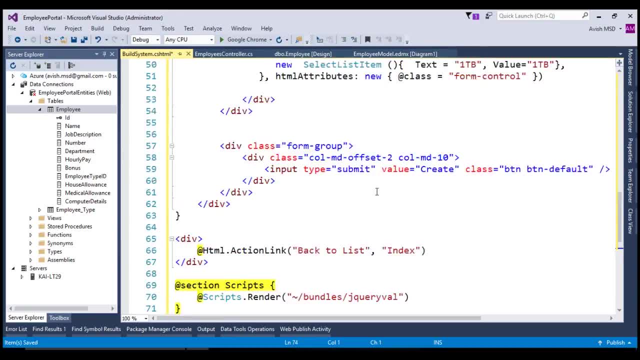 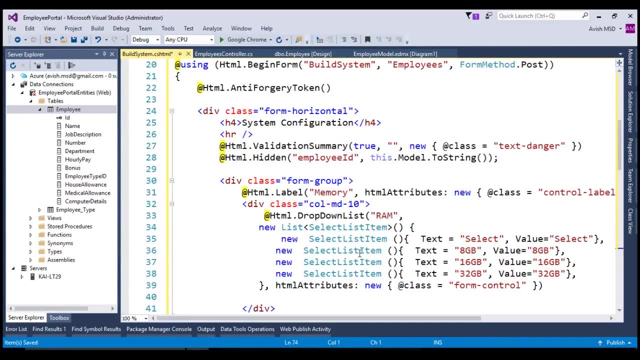 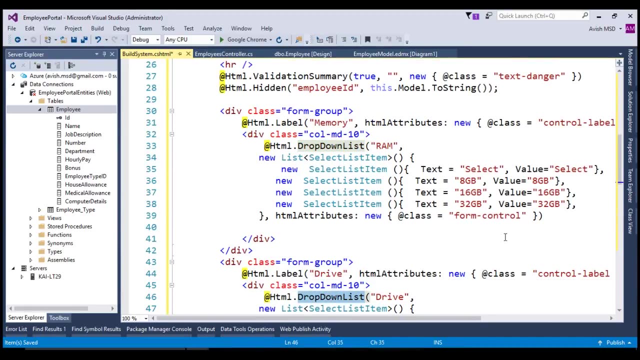 Let me just copy that code over here Now. if you notice the code, I have already created two dropdown lists. I will use this to choose the value of RAM and hard disk drive. Further, while configuring the system, user can opt for 8GB, 16GB or 32GB as the memory. 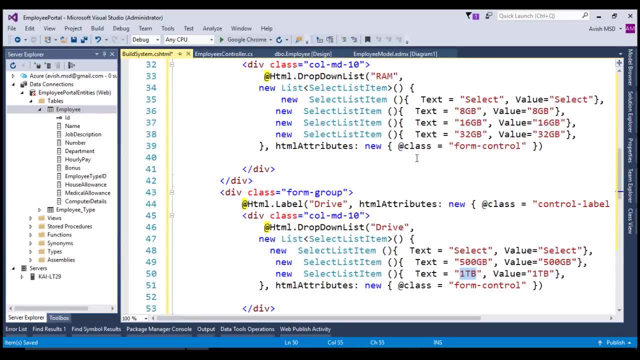 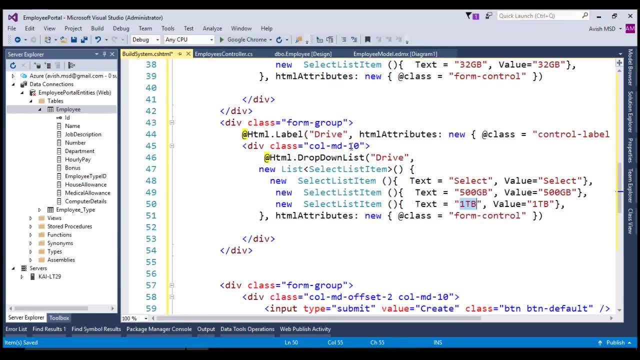 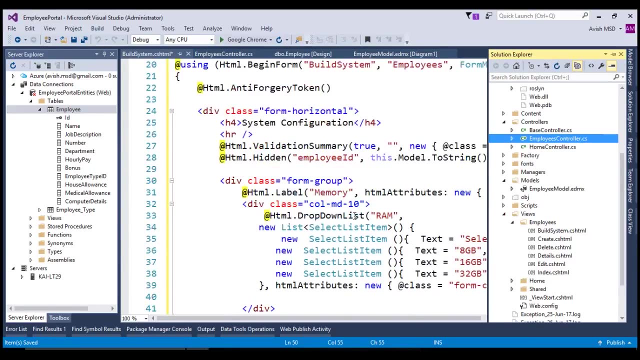 and 500GB or 1TB as the hard disk size. As we progress by, I will add more configurations to build a system. Let's now switch back to the employees controller And add a new action method so that we can capture all these details on the form submit. 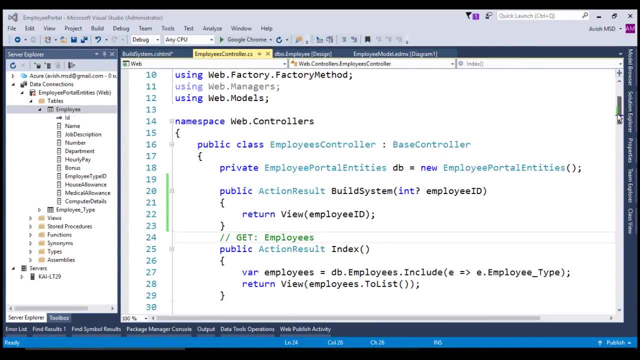 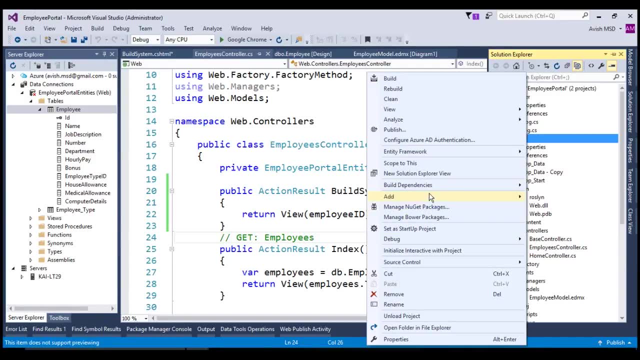 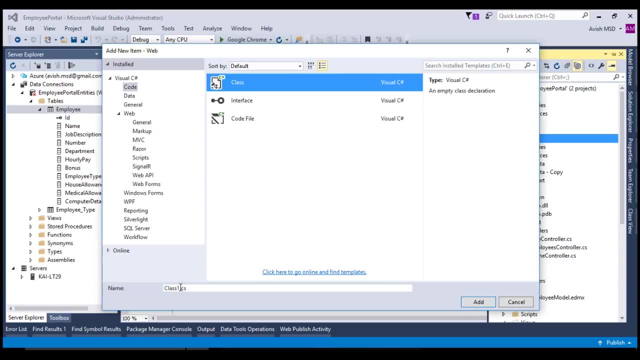 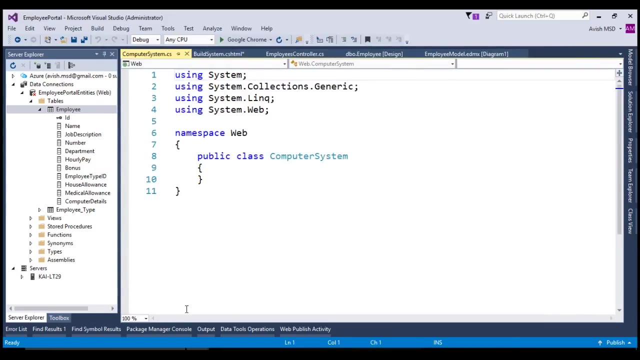 Let's switch to the employees controller By creating an action method. let's create a new class, Right click on the web, add new item and choose a class under code, and let's name this class as computer system. We are calling this class as computer system, since we are going to configure the details. 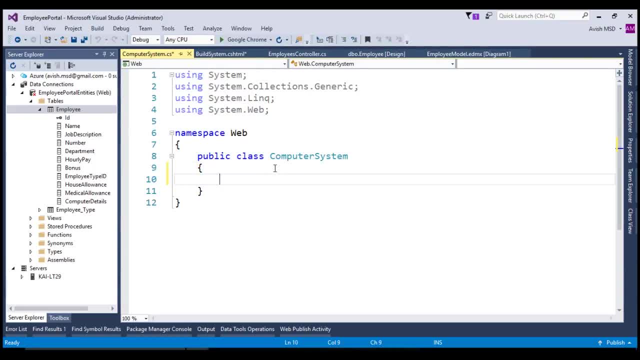 of the computer system. Let's add some properties which would be private string and name this property as underscore RAM, private string underscore HDD size as another property, Let's add some properties to capture the hard disk size. Let's add some properties to capture the hard disk size. 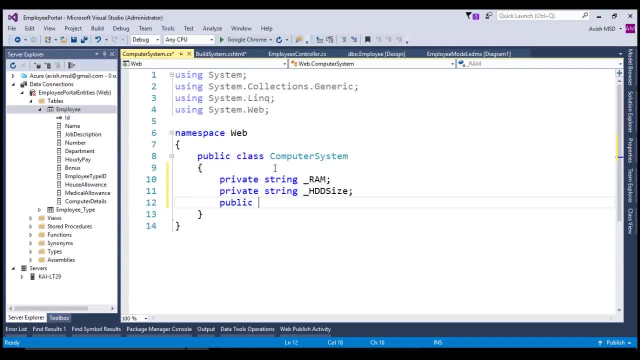 Let's add some properties to capture the hard disk size, drive size which is chosen, and let's create a constructor, public computer system, a public constructor as well as another constructor which accepts the parameters of RAM and hard disk drive. let's assign these values to the 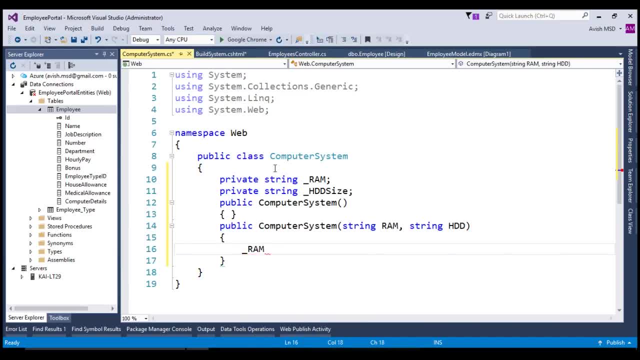 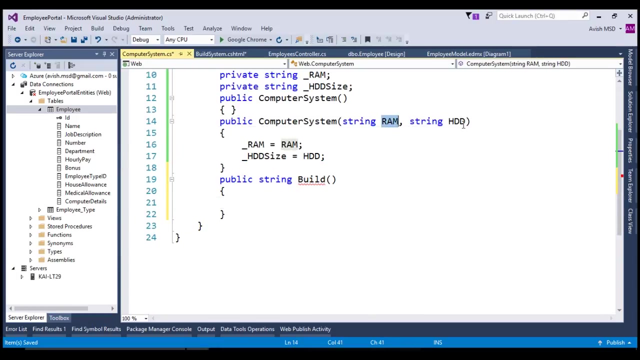 internal properties saying: underscore RAM equal to RAM. underscore hard disk size equal to HDD. let's also create a new method: public string build. let's name this method as build, so that it's going to build the system by using the RAM and hard disk size that is being passed into this. constructors. let's 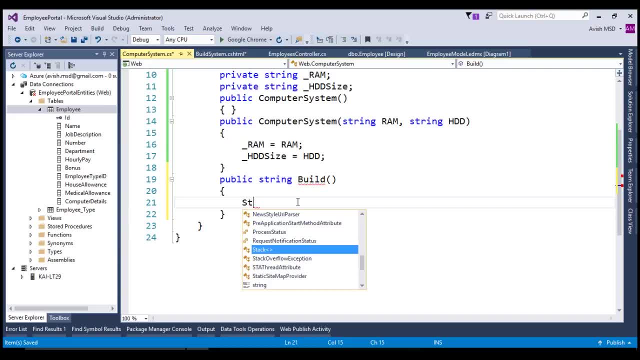 create string builder as B equal to new string builder. let's resolve these issues by using system dot text and let's say SP dot up in string dot format of, let's say, RAM colon, zero comma underscore, which is assigned in the constructor. similarly, let's do the same. 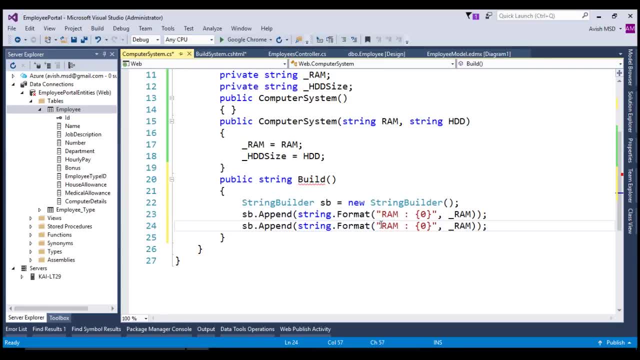 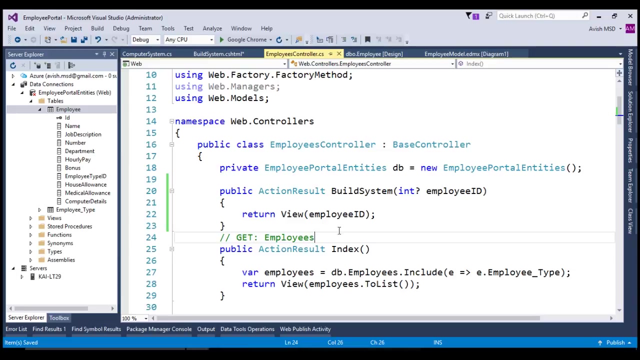 thing. with the hardest type it should be HDD size equal to underscore HDD size. now let's return SP dot to string. let's now switch back to the employees controller. Let's now switch back to the employees controller and let's say that the create our action method to build the system. the previous action method would 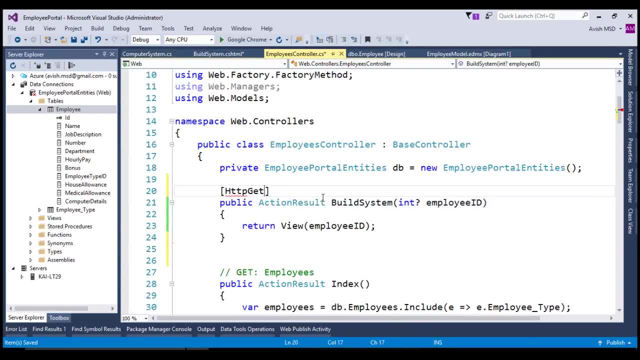 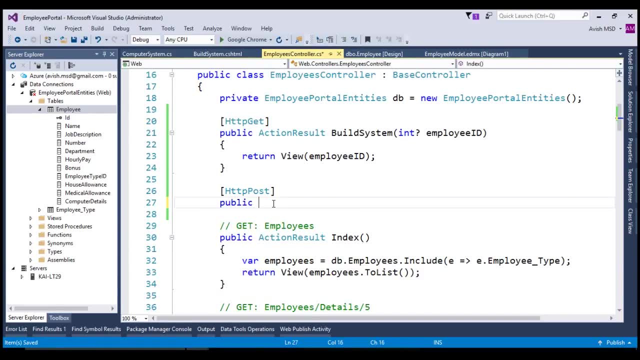 be a HTTP get, whereas the submit action method would be a HTTP post. let's create the action method public action result and the action method name would be build system, which accepts the parameter as employee ID comma memory that is being chosen in the view and it passes back the hard disk drive size that is chosen. 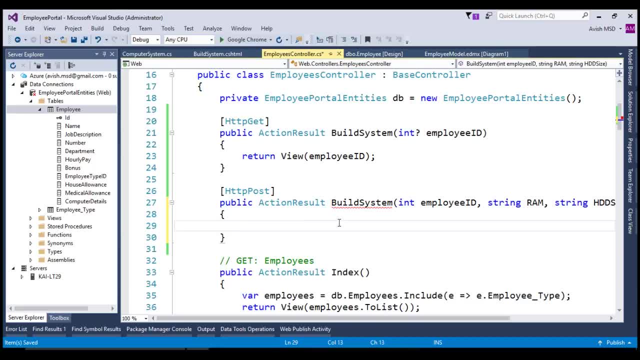 from the view based on the employee ID that is being passed. let's retrieve the employee object from the database- let's say, employee equal to DB, dot, employees, dot, find- and let's pass this employee ID as the input parameter to the find, now that we retrieve the. 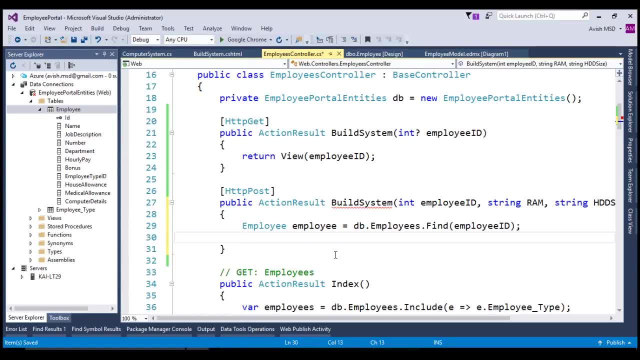 employee. let's build the system. let's initialize and instantiate the class computer system equal to new computer system. what is that? the computer system has got two constructors accepting the input parameters for RAM and hard disk drive size. let's pass the RAM comma hard disk drive size as well, now that we have retrieved 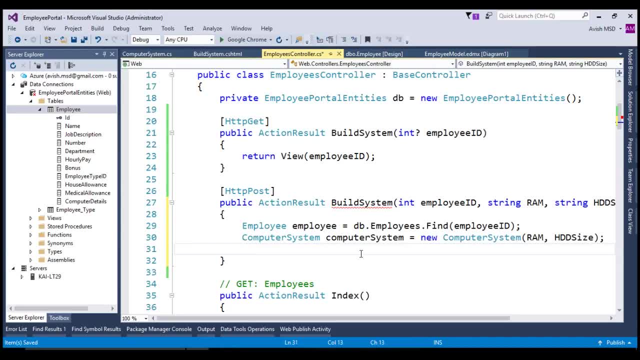 the employee details assign the system configuration. using this computer system class- let's say employee dot. system configuration details equal to computer system dot built- the build method will retrieve the system that is being built and it gets inserted into this system configuration details column. now let's say we need to update this employee object back to the database. so let's say db dot. 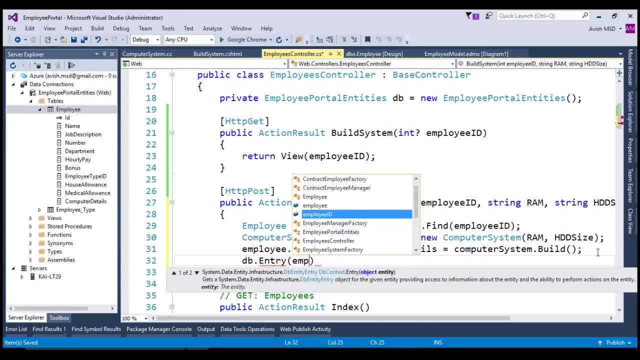 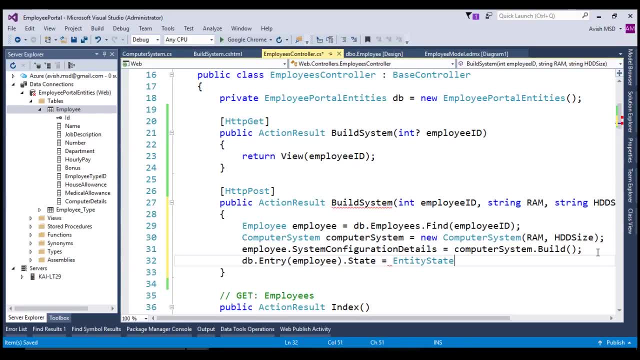 entry. let's create an entry for this employee object with a state which is entity state dot modified. as we are modifying the employee back to the database, let's say db dot- save changes. to save these changes to the database, table 1. we have successfully saved the changes. let's redirect the view to the index view by using: 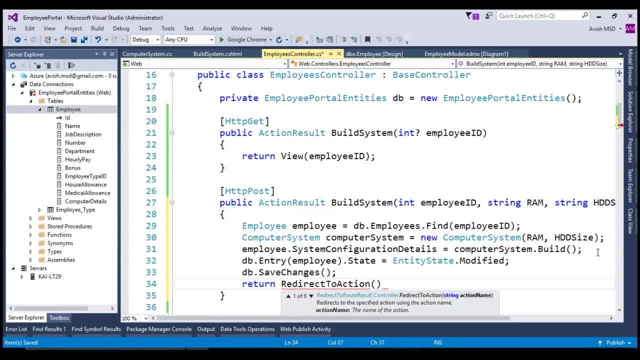 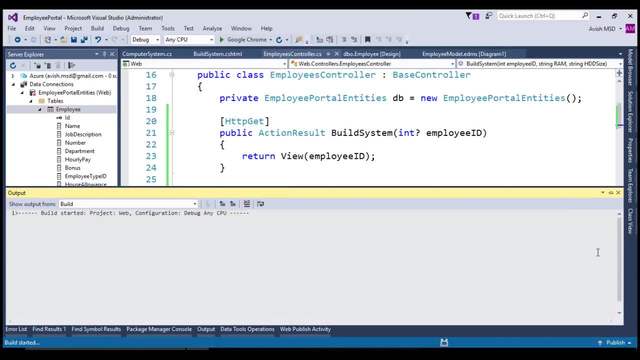 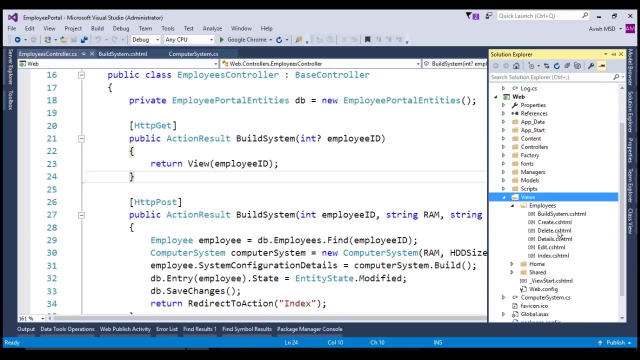 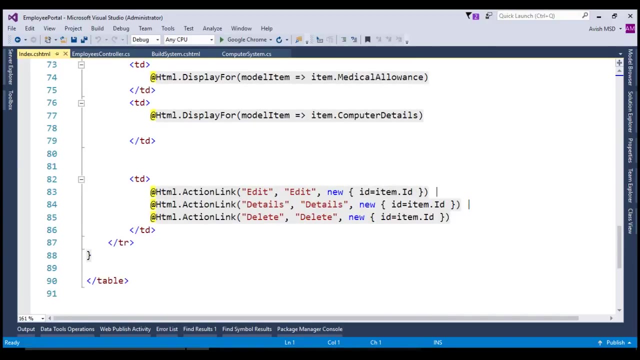 redirect to action and let's pass index as the parameter. let's compile this application. look at that. compilation succeeded. let's now switch to the index view. let's open the views and choose index view and add an action link to configure the system. let me just copy the link that have it in my notepad. 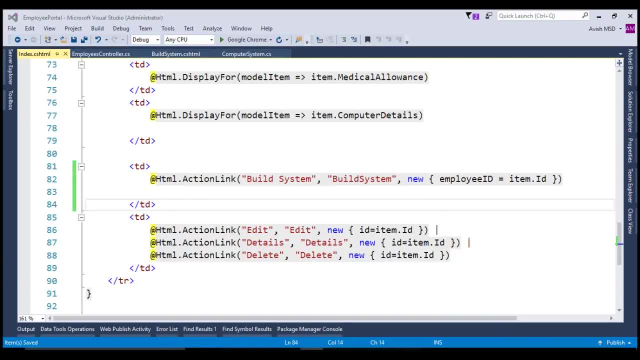 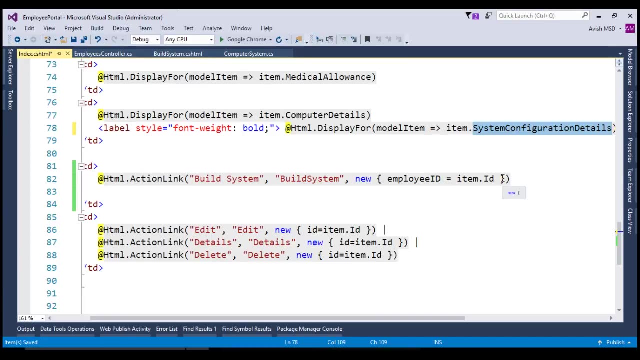 now let's also create a label to display the chosen configuration details. let's keep that label over here after the computer details. so if you take a look at this, we are displaying the system configuration details that are already configured for the existing systems. let's switch to the employees controller and run this application. let's click on the employees tab. 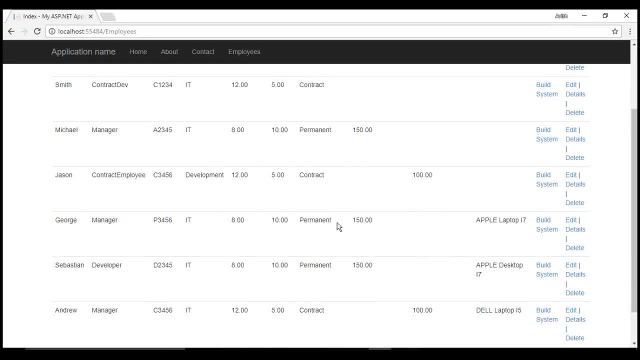 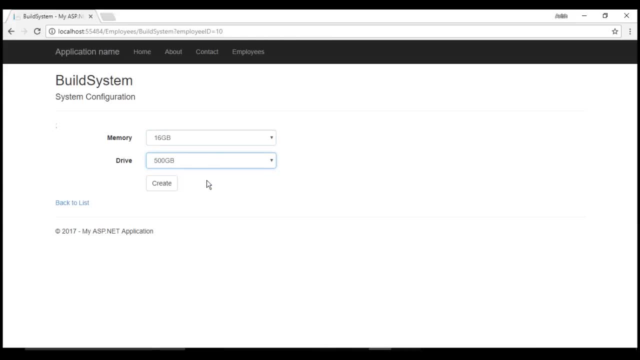 out more information about the mobile person and the system which you are targeting now to be used as mobile, let's click on the building system module, where we will start configuring andmesias system, which you all know of job brain and chooseام하세요 הוא했습니다.